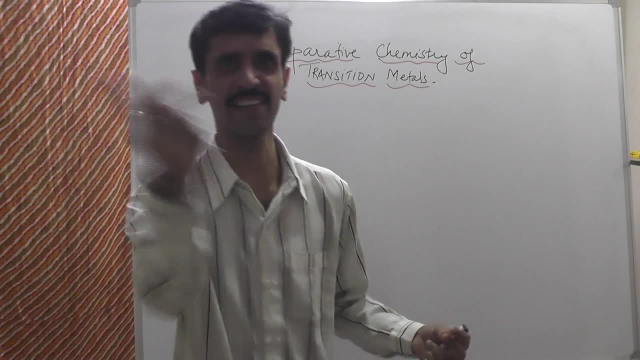 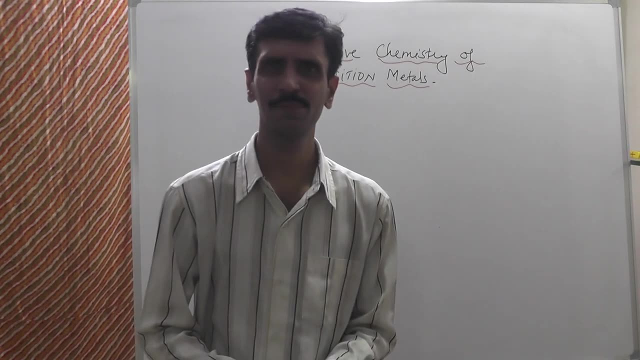 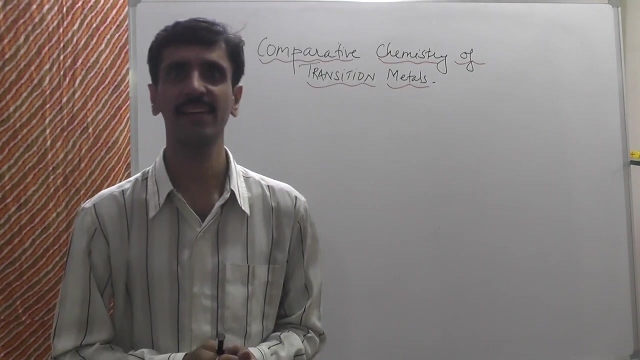 the basics are very strong, the advanced level becomes very easy. all right, so the basic of inorganic chemistry, everybody will understand, and that is periodic table. what is periodic table? its a systematic classification of elements. now, when I used a word systematic, then in oratorics our mind, because we have to have a 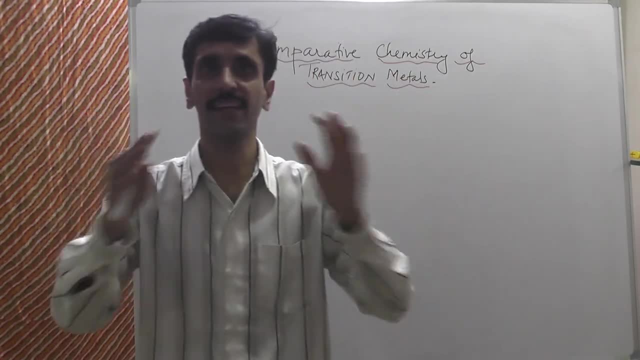 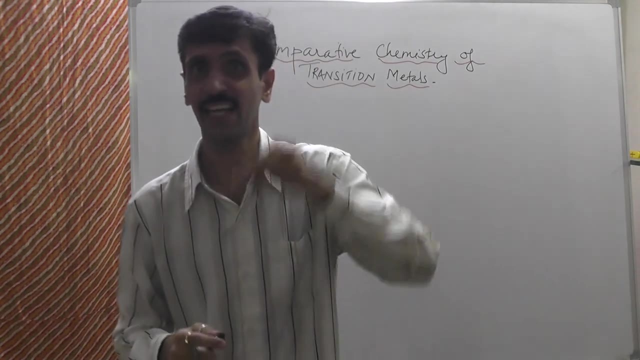 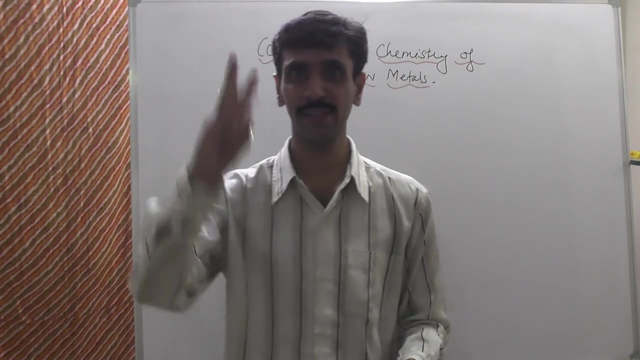 constituent parameter in our mind which refers to the actual classification. That parameter is the final electron entering into which particular organ. respectively, There are four orbital under consideration: s-orbital, the p-orbital, the d-orbital and the f-orbital. So the last electron entering into that particular, 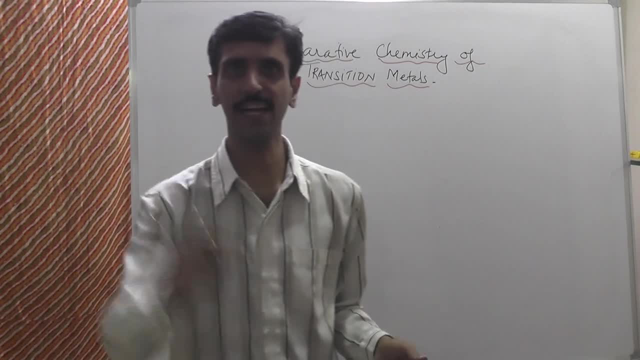 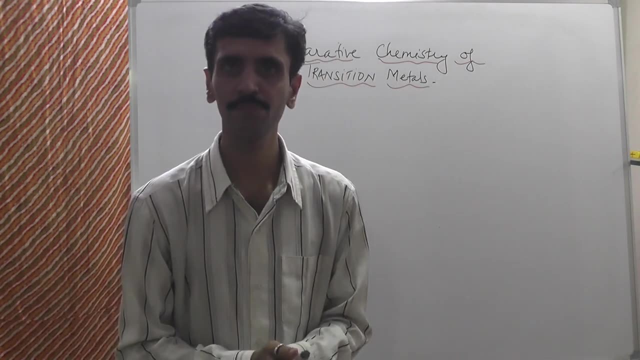 orbital, that block, it is called as. So if the last electron goes into the s-orbital, then it is called as s-block. Similarly, we can talk about p-block, d-block as well as f-block. I guess this parameter is very clear. Next, what is the skeleton of a periodic table? 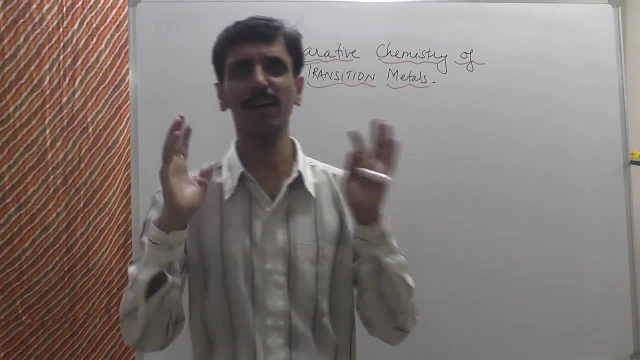 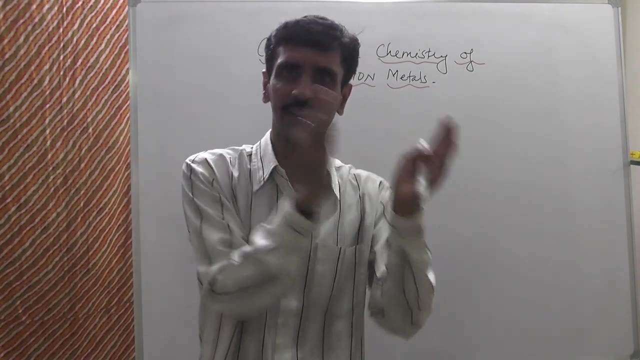 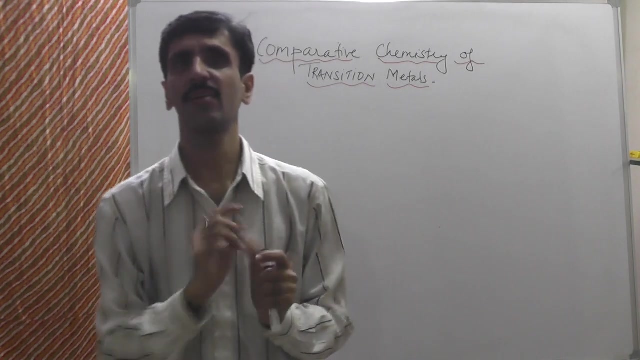 How the elements are arranged, The positions, how they are. So for understanding that, let us try to go to a very simple part, and that is s and the p are metallic and non-metallic respective. Here I would like to say all p-block elements are non-metallic. Okay, it's. 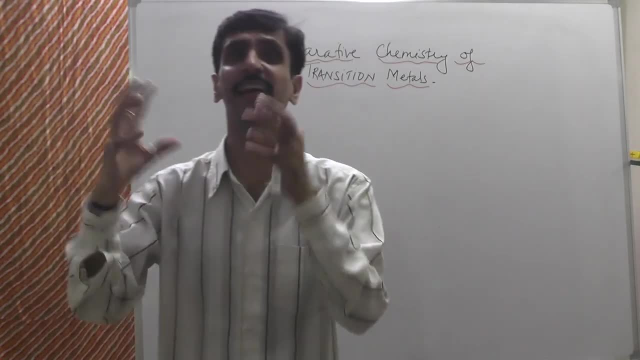 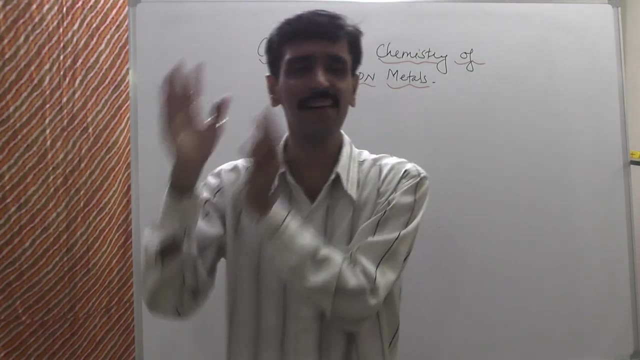 a mixture. Some of them are non-metals, some of them are metals and few of them are metalloids, showing a metallic as well as non-metallic character, both. But then generally we consider p-block as non-metals, s-block as metals. So they are, both of them are opposites. So 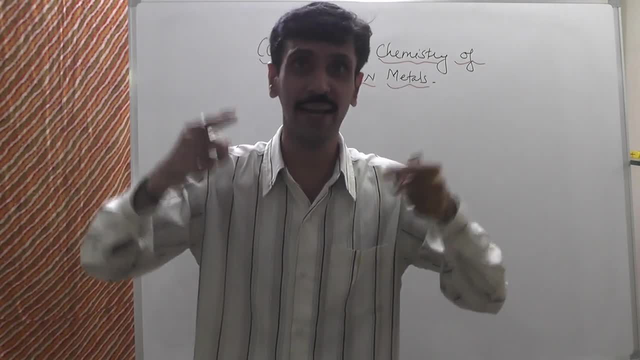 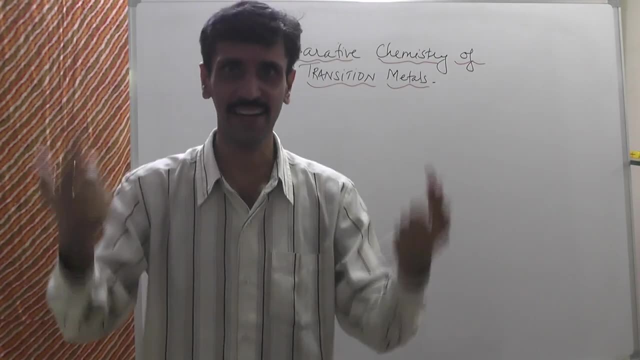 just consider- okay, I am just giving you a trick- how to remember the positions of the various block of elements in the periodic table. So just try to consider that trick. and that is, imagine that s and p, both of them, are enemies, and if both the enemies are, 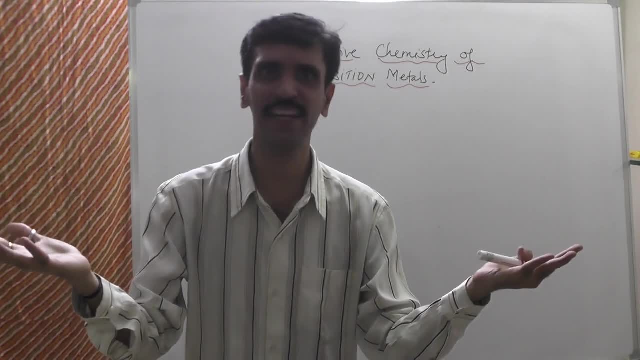 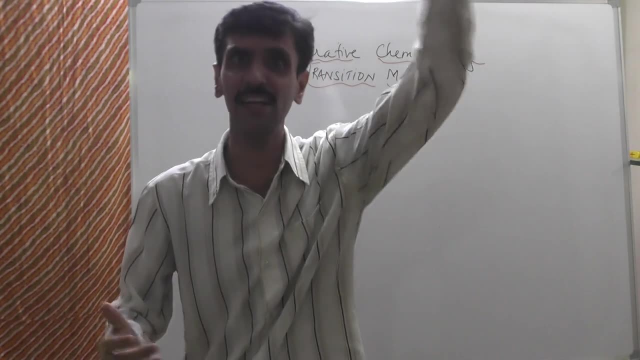 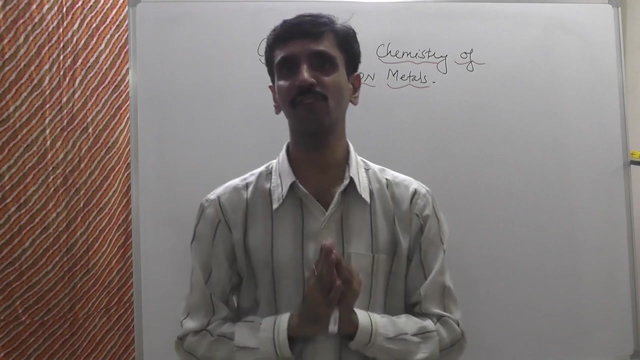 together, there will be a fight. there will be a fight. instability And periodic table is stable because it is existing since many years. hundred and fifty years, we completed our periodic table. be knowing this, then, for stability, what has to be done is these two enemies has 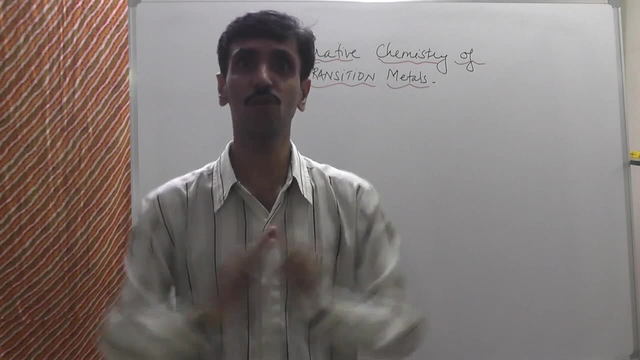 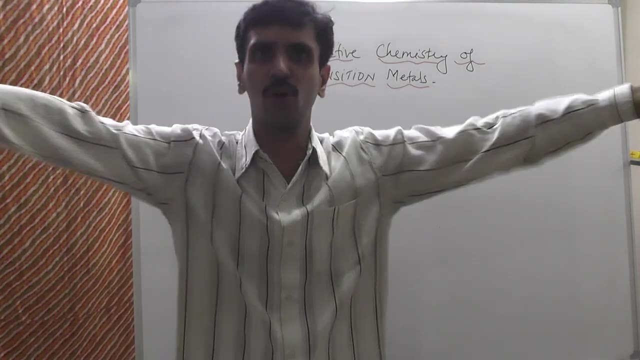 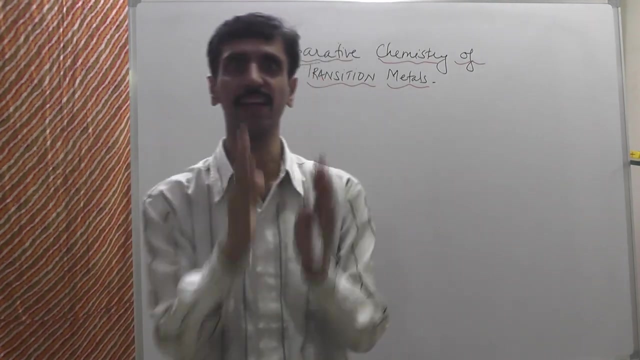 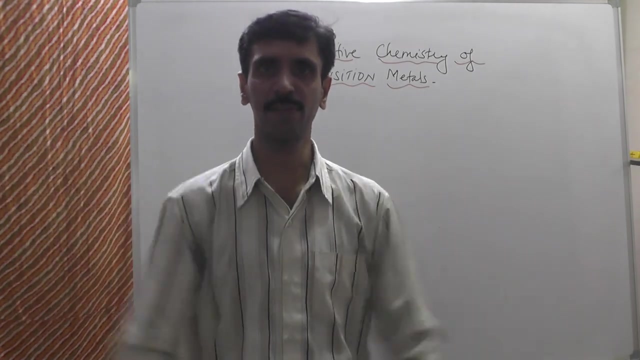 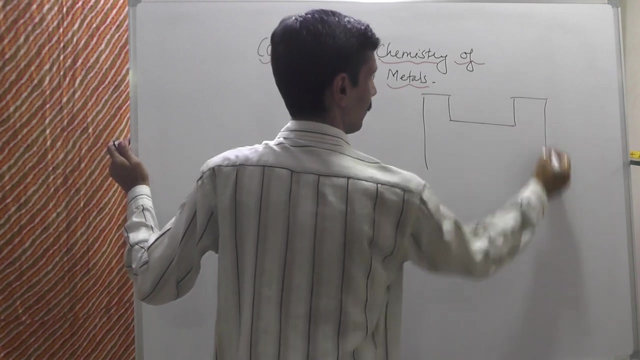 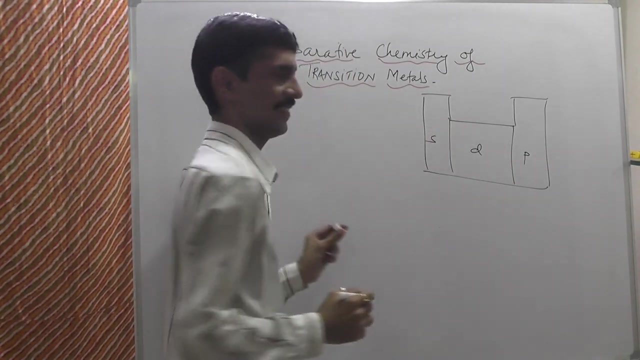 to be kept aside. all right, so the arrangement will be like this: so S on one side, the P on the other side, and in between comes what D. the next thing is: in a classroom also there are some character students. okay, I hope you understand what is what I mean. 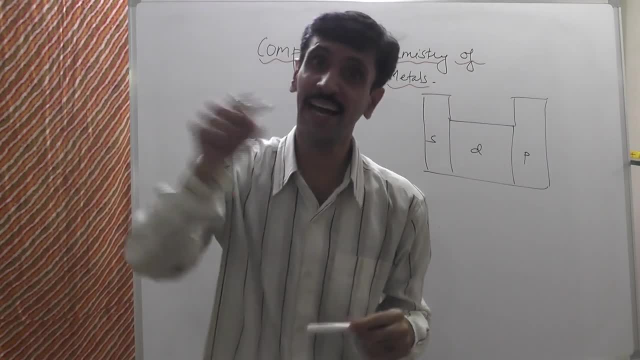 is especially sitting with the last majors. all right, they are the part of that classroom, but the characters are different. all right. so what we need to do is, in order to make sure that our lecture goes well. we need to make sure that our lecture goes well. we need to make sure. 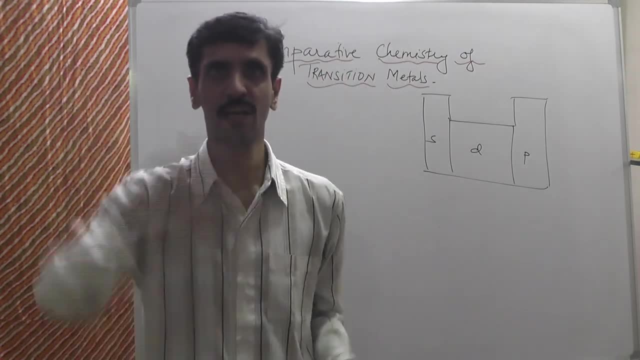 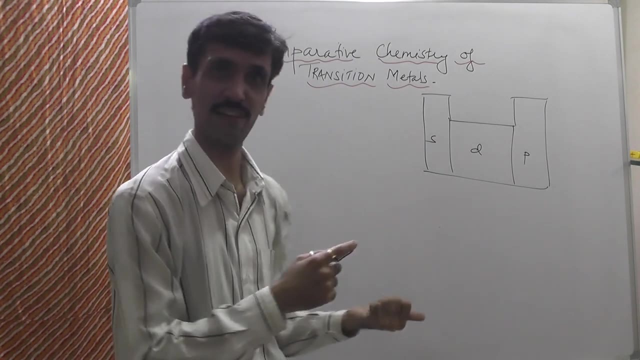 very smooth. we need to change the position of that particular student, bring into first bench and things like that. all right. so that means what we are changing the position. same thing is for F block also, F block elements are a part of D block elements, but because the characters, because their properties are, 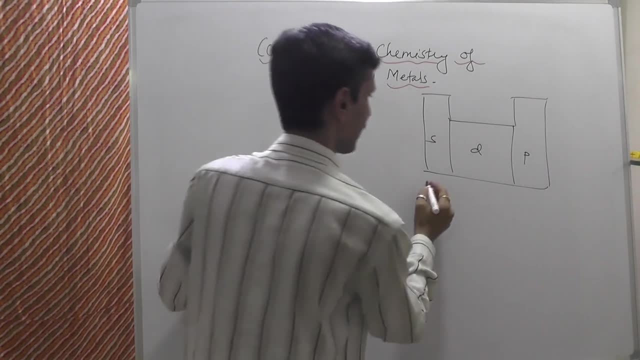 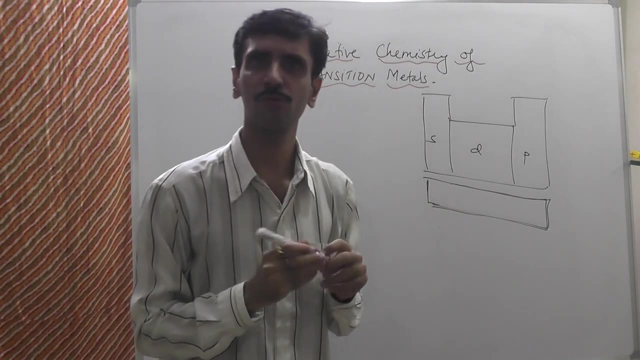 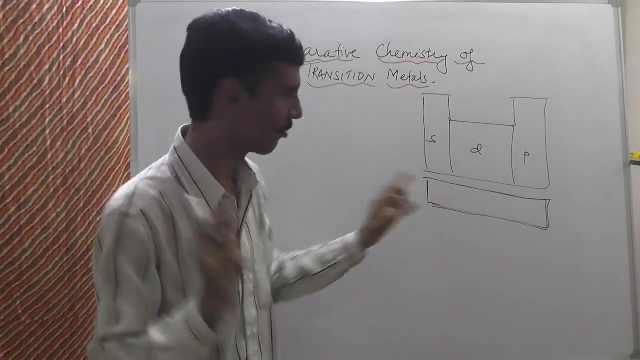 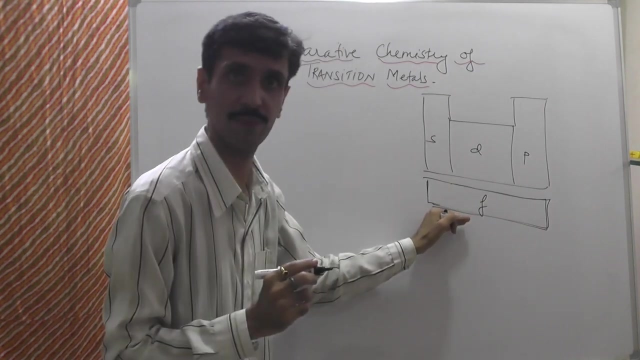 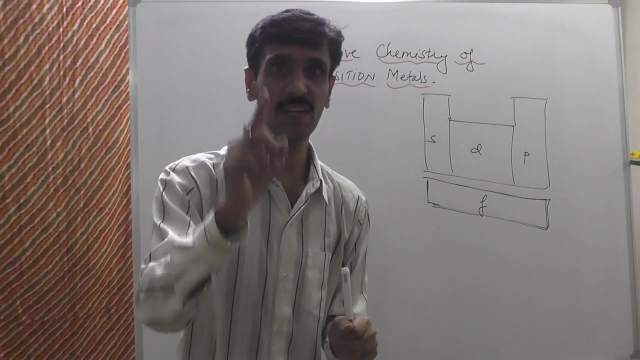 different and therefore we give different position and that is going to be at the bottom of the periodic table, absolutely aloof, so they're not going to interact with anyone, okay, okay, so that means you know the capacity is of all these are videos. maximum capacity: okay, s2, P is 6 and t is 10. so whatever is the maximum capacity of the. 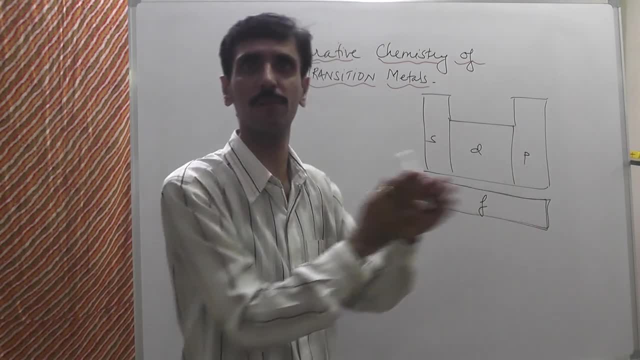 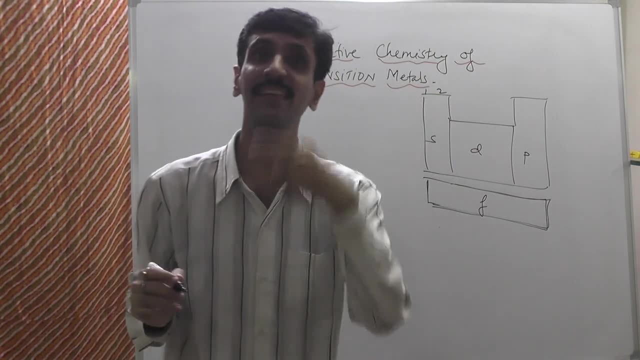 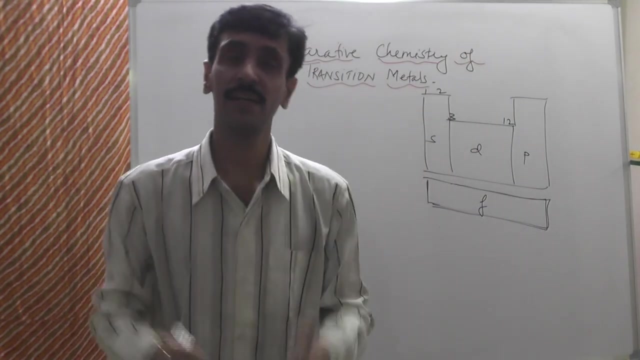 orbital that many groups are being assigned to that particular block is 2, so therefore group number is 1 and 2.. After that D comes. D's capacity is 10, so 10 groups are assigned to this and therefore it goes from 3 to 12.. For P the maximum capacity is 6, so 6 groups are assigned. 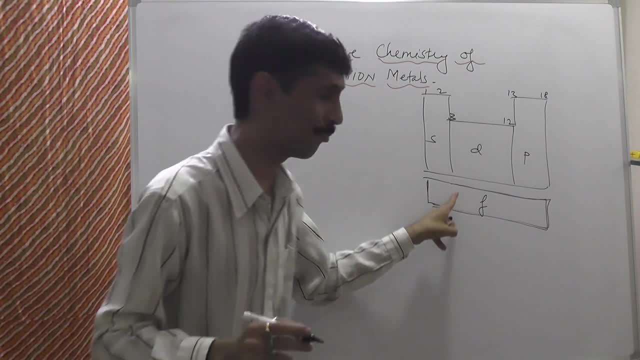 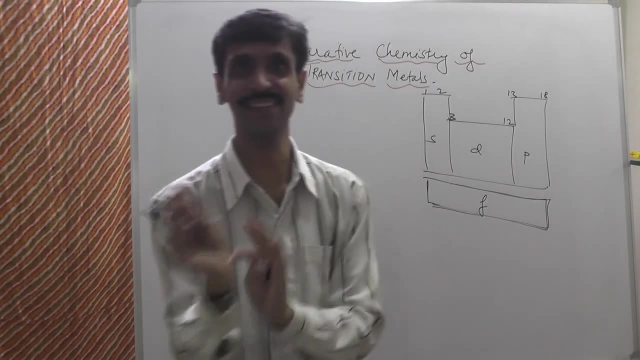 so that is 13 to 18.. Okay, I won't give 14 over here. I have already given you the reason why it is so. yes, okay, that is, they are not different. they are a part of D, but only the characteristics are different. 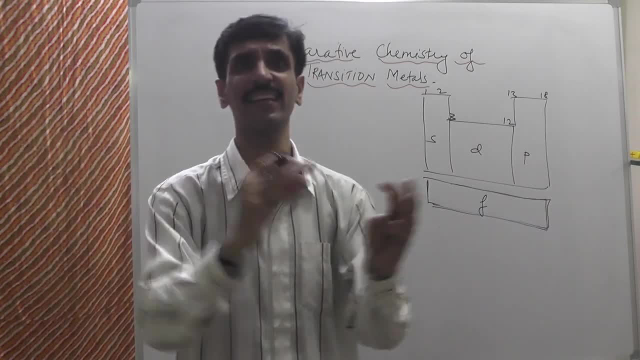 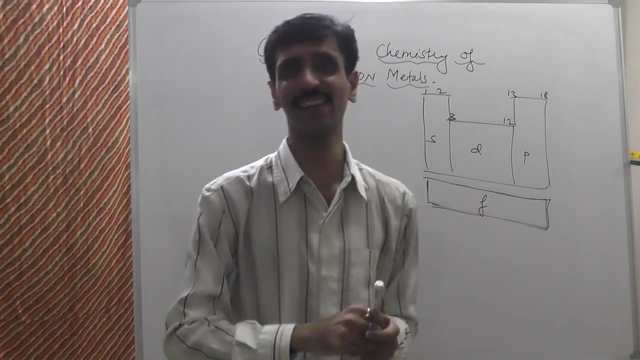 so, therefore, we are giving different positions and therefore, if you add all these, you come to know that there are 18 groups in the periodic table which you have been learning now from a long time, ever since you have started learning chemistry. Alright, so this is the way we get this. 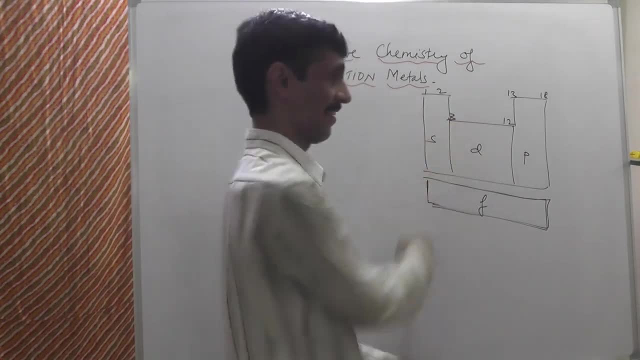 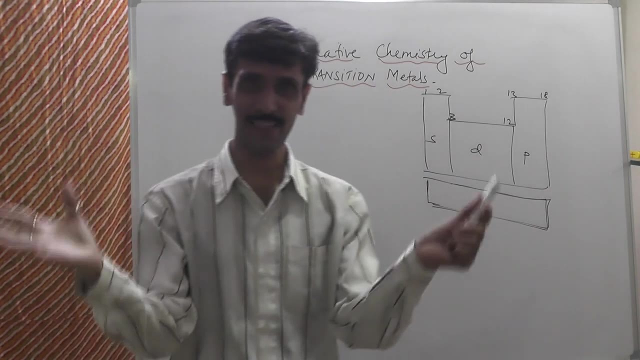 18 number. it is not a magical number. this is the technical reason why we have 18 groups in the periodic table. Alright, so this is the introduction part about what exactly the periodic table is all about. Now, as I said about the properties, the position of the elements are related to the properties. 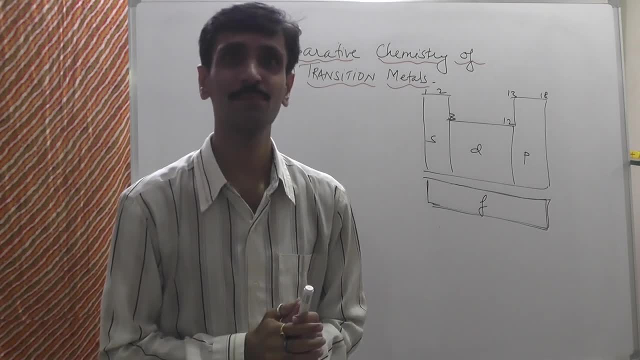 Alright S block. all the S block elements are related to the properties. Alright S block. all the S block elements are related to the properties. And the P block, as I said, is a mixture of metals, non-metals, metalloids. 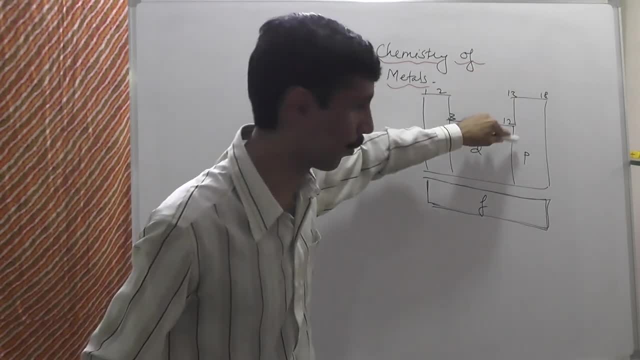 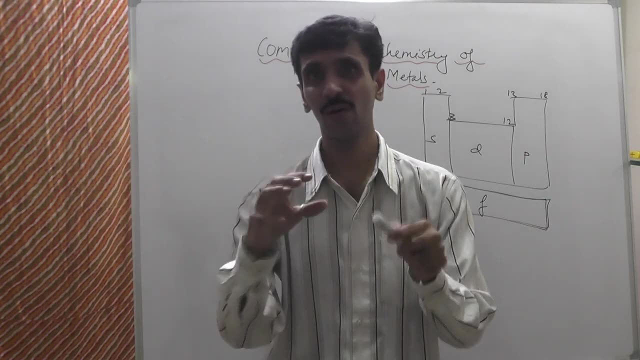 Okay, the top ones are going to be non-metals, the middle one is metalloid and the bottom one are metals. Okay, that is what is the arrangement of the P. block elements are Alright. so now what happens is: overall, we consider it is non-metallic. 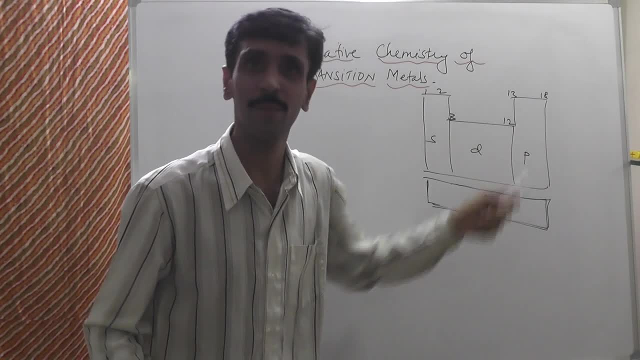 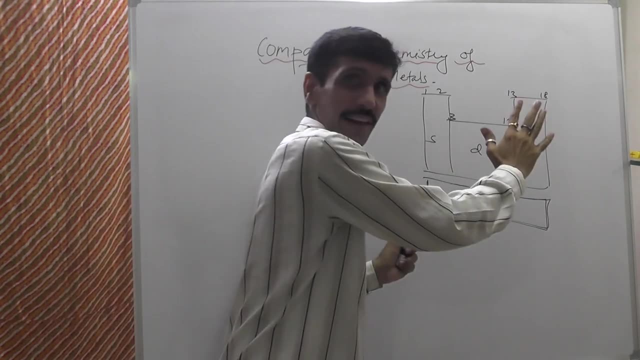 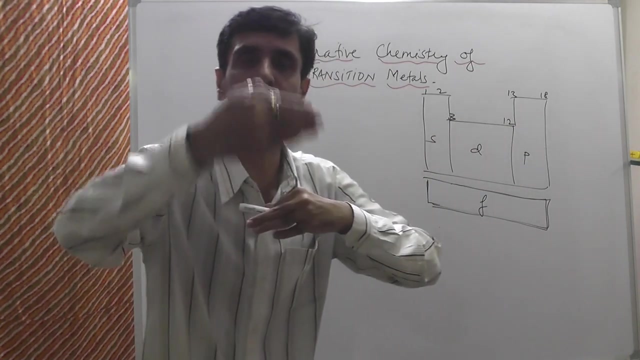 because even if they are metals like lead and tin and all that, but they are metallic characters as compared to S block is less Alright. so that is why, overall, we consider general impression. We consider it as non-metallic. this is metallic. Okay. now there is a changeover, because metallic and non-metallic properties are opposite. 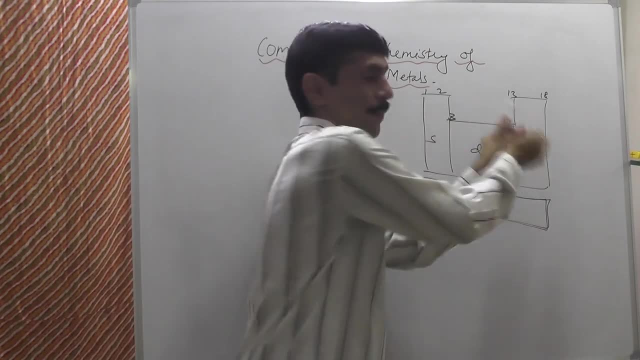 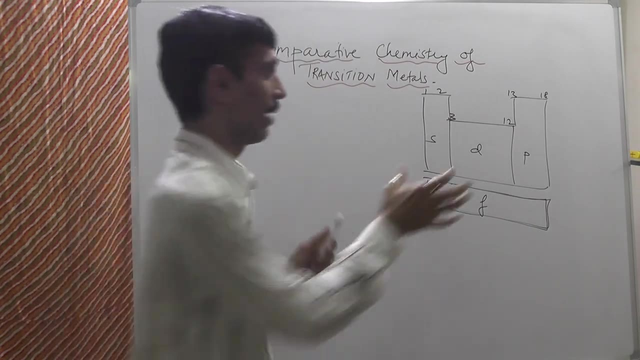 You also know this. So this changeover is going to happen when we go towards S and P, From a metallic character to a non-metallic character. But see, friends, how this changeover is happening. Because this changeover is taking place through what? 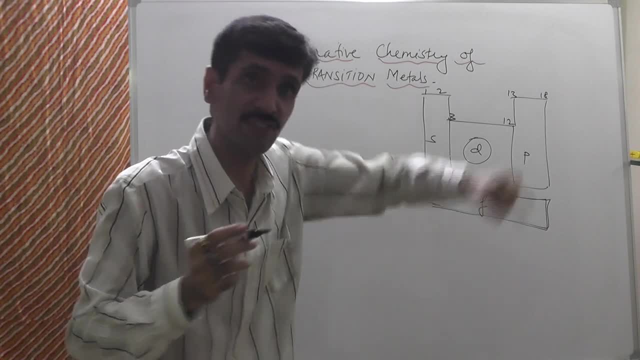 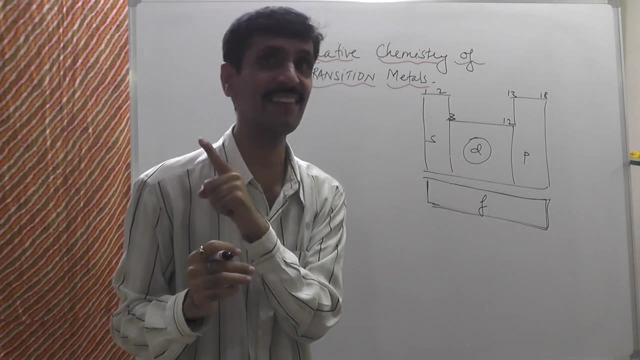 This D- Okay, it is taking place through this D- and D has got 10 groups. So what we say now about this changeover? It is a gradual change or a sudden change. Oh yes, I can hear it. You are saying it is a gradual change. 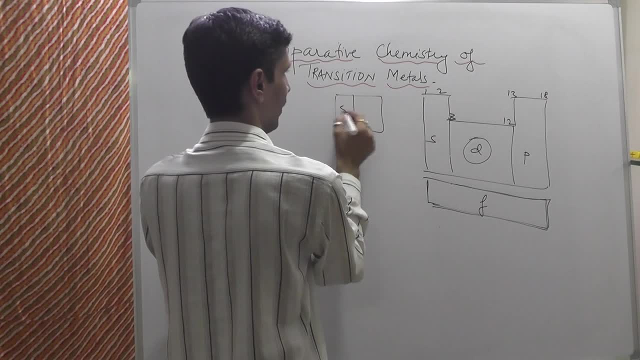 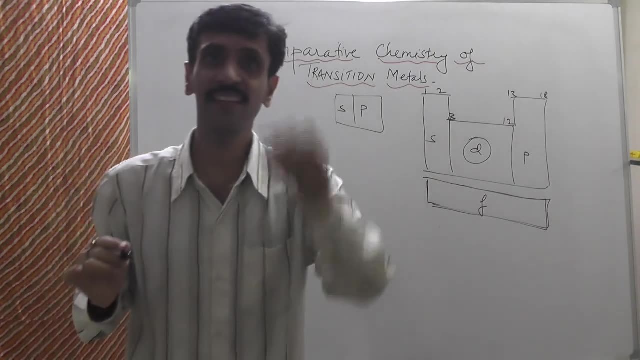 Now, if S and P- I have shown like this: This is S and this is P, Then I would have said it is a sudden change. But here there is a D. Okay, so this D is representing that. yes, it is a gradual change. 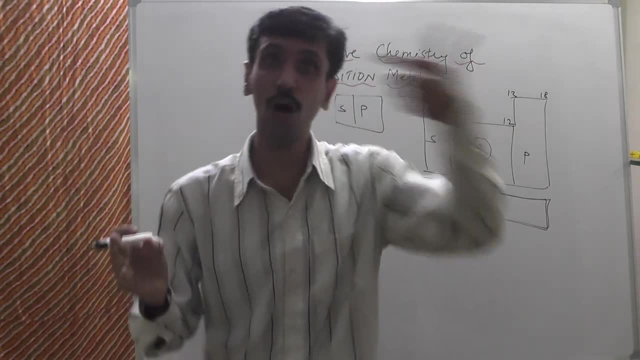 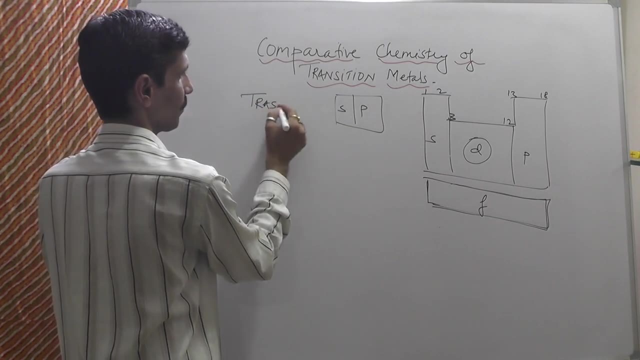 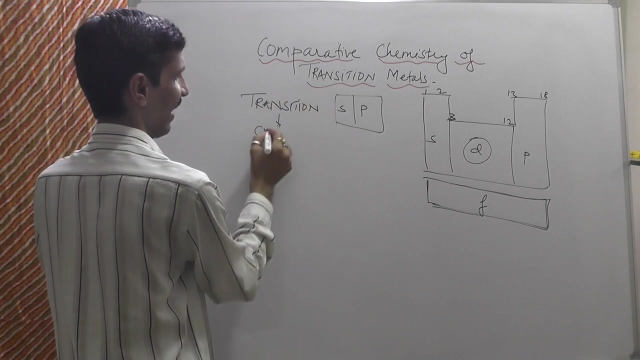 Okay, this gradual changeover, Okay, between the two opposites is called as what Transition. Now you must have heard: Okay, it is called as what Transition. So this transition is a thing, but it shows a changeover phase. 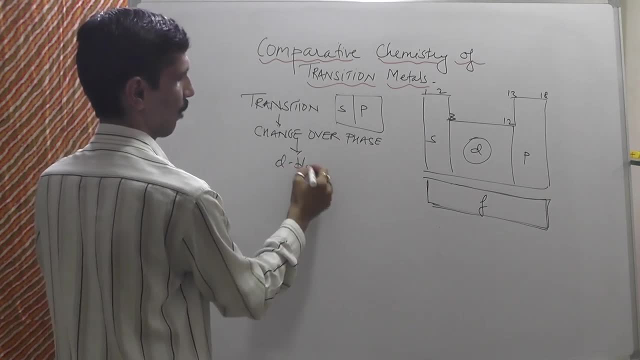 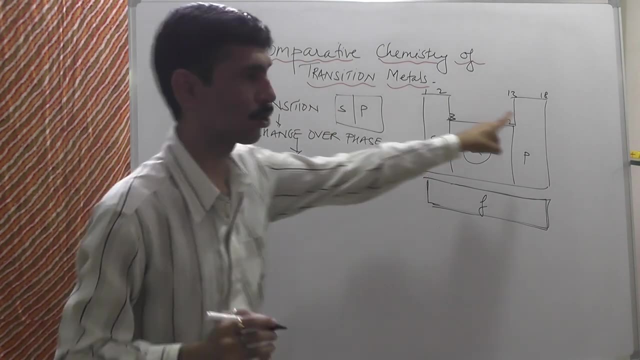 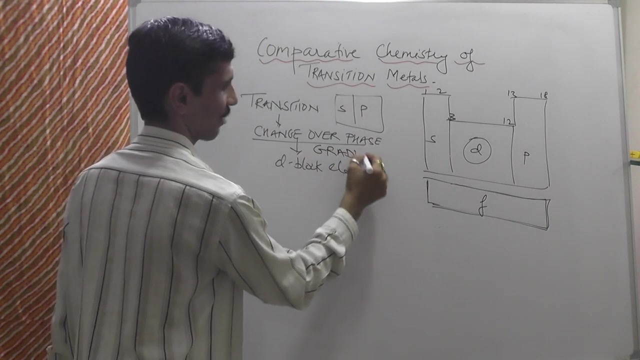 Okay, and that is what are being shown by the D block elements. Okay, changeover from a metallic character to a non-metallic character. And this changeover, Changeover phase, is what? Yes, it is gradual, It is not a sudden one. 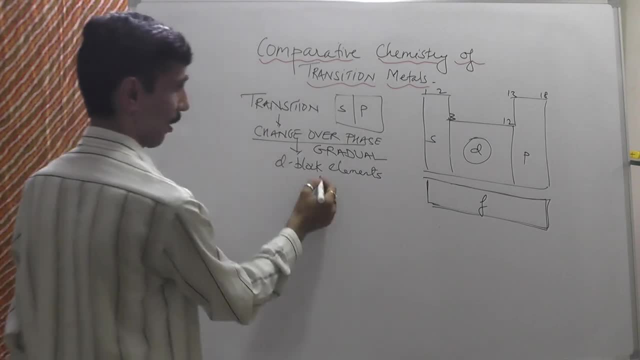 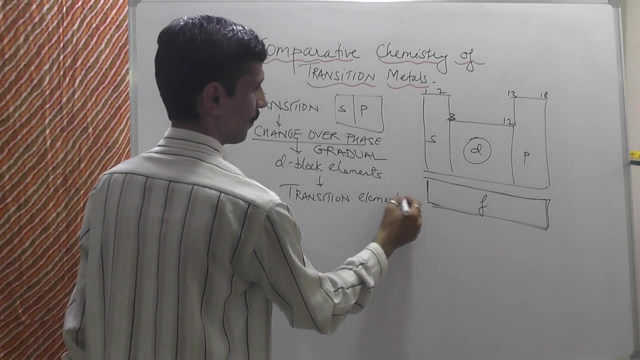 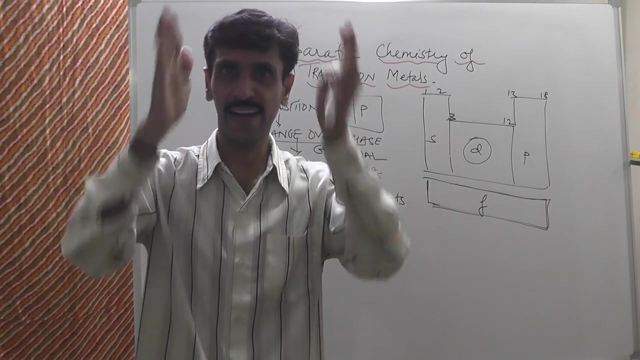 Okay, and that is what is called as what? Transition And hence D block elements. they are called as transition elements, So, as a result of which, in a lecture also, you have to be completely focused on what the teacher is teaching. Okay, our entire attention has to be centralized. 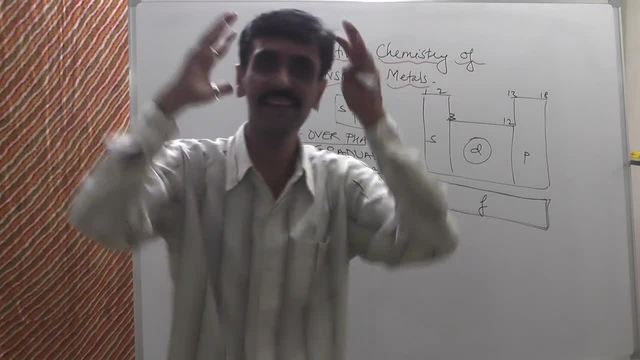 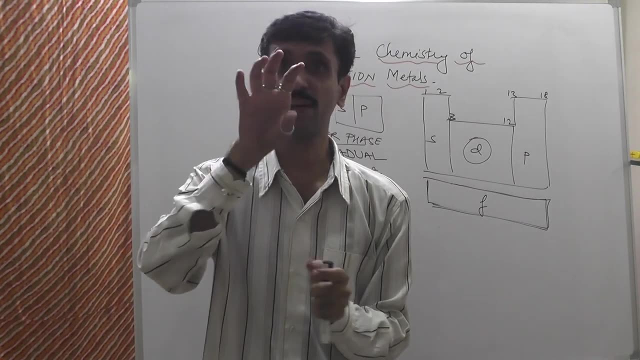 Same thing is over here in this particular chapter also. So our entire focus is on this center. Okay, that is, D orbitals. Okay, in this entire chapter we are going to consider those Okay D orbitals, the D block elements. 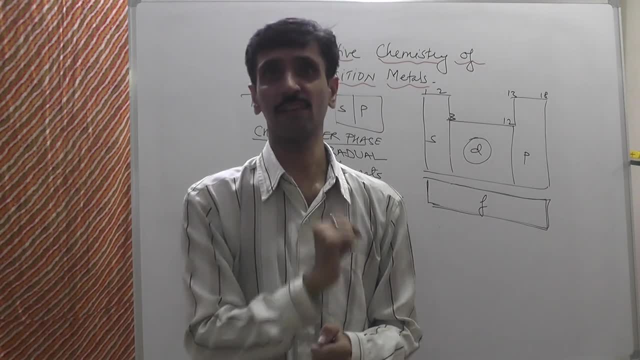 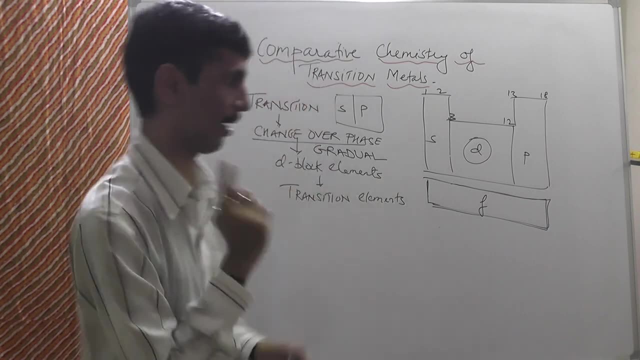 Okay, and because they are going to, once I say, significance of a gradual changeover from a metallic character to a non-metallic character. Alright, and those are D block elements. So I hope you have understood up to this far. 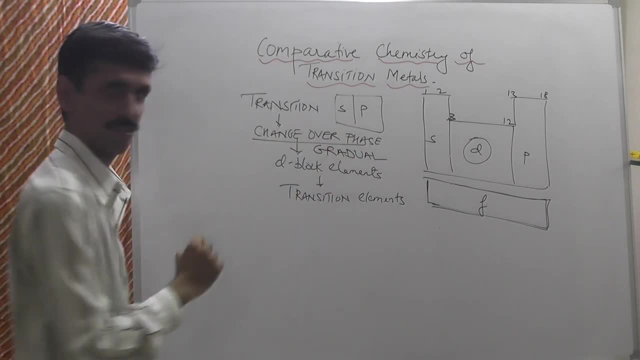 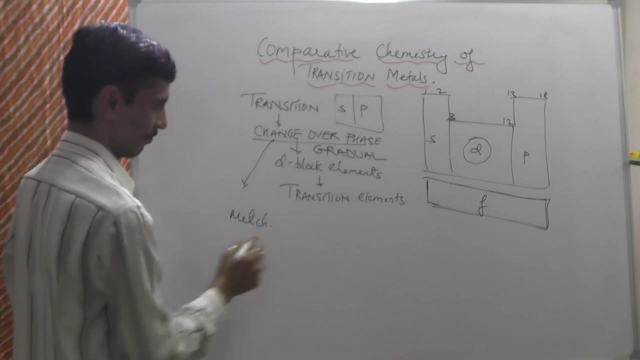 Transition means what It is: a gradual changeover phase. Okay, so here the changeover. What kind of changeover is going to take place? What kind of changeover is going to take place From a metallic character that is nothing but S block to a non-metallic character? 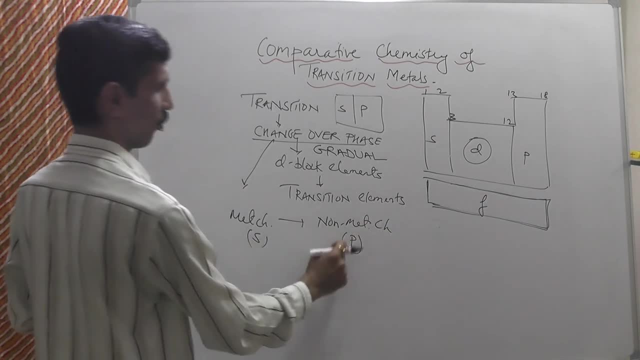 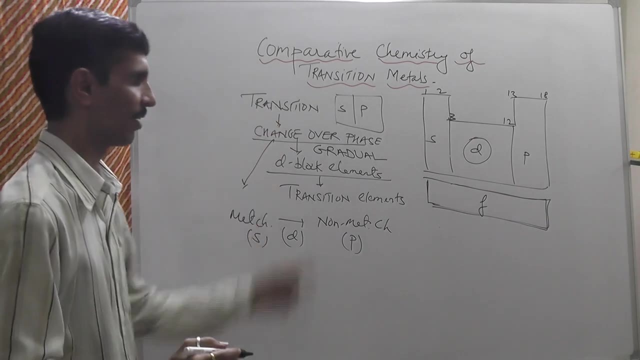 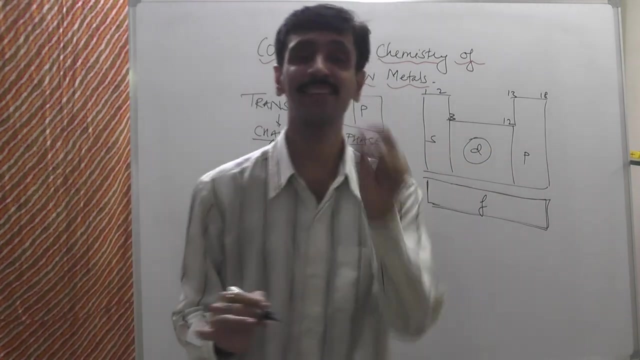 Okay, and that is P block. So this changeover is taking place through the D block elements and therefore these D block elements are being called as what? Transition elements? Now, all these D block elements, all these are metals. Okay, are what? 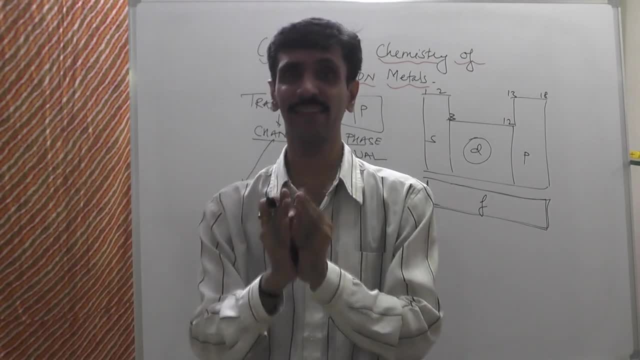 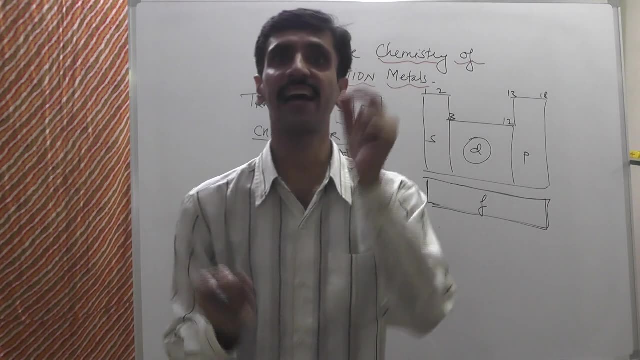 Metals. Once again, I repeat: all D block elements are metals. And when I say D block elements as transition elements and because they are all metals, so I call it as what? Transition metals. Okay, there are many of them, So from group 3 to group 12.. 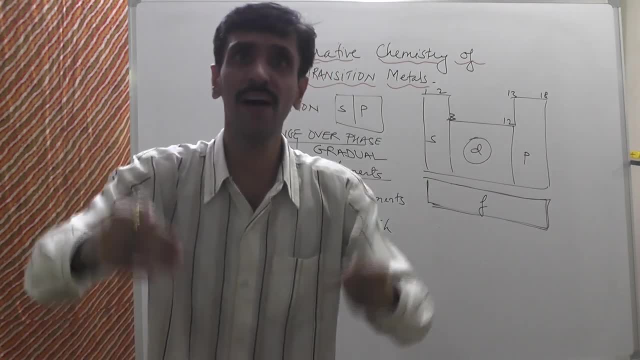 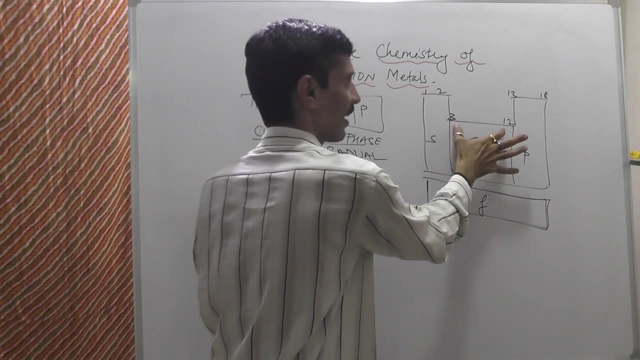 So there are many transition metals And we do a systematic comparison of the properties of those transition metals. Okay, from group number 3 to 12, what is happening? As I said, we are going to completely Focus on the center. 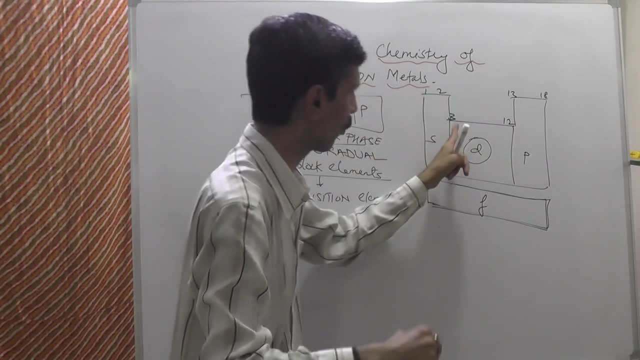 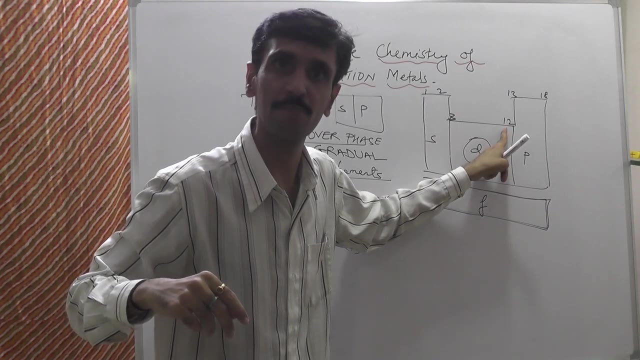 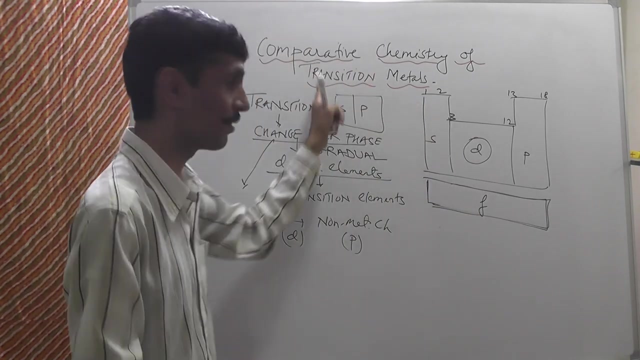 Okay, so what is the changeover taking place of the properties as we go from group 3 to group 12?, That is, as we go through the first transition metal to the last group transition metal. Okay, and this is called as comparison and hence the title of the chapter is Comparative Chemistry of Transition Metals. 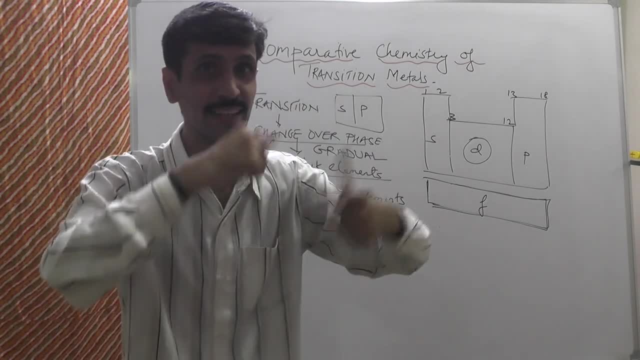 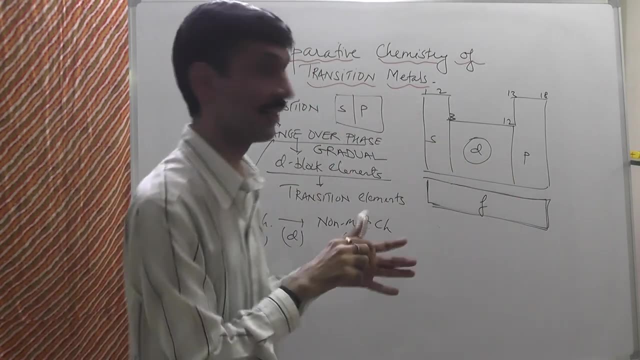 Please be very careful. The comparison is taking place only within the transition metals. I specified it's group 3 to group 12.. I'm not comparing this D block. I'm not comparing this P block with the S block. Neither I'm comparing it with P block or F block. 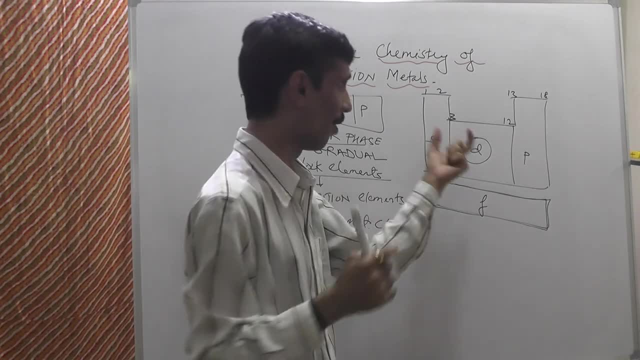 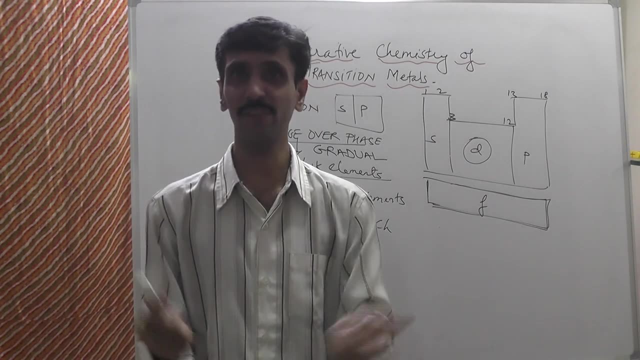 Be very clear. I'm making a comparison, very clearly, amongst the transition metals itself. Alright, so this is what the title is. We are making a comparison of the properties of the transition metals. What do you mean by transition metals? You understood this very well. 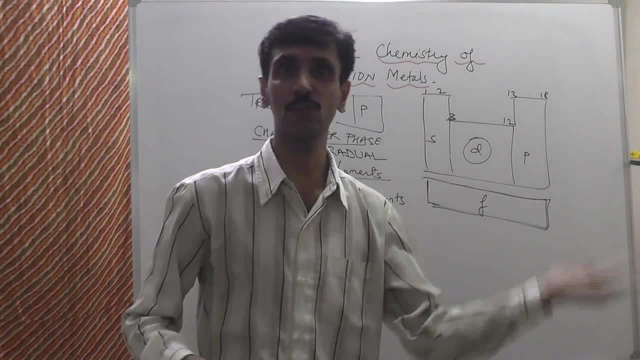 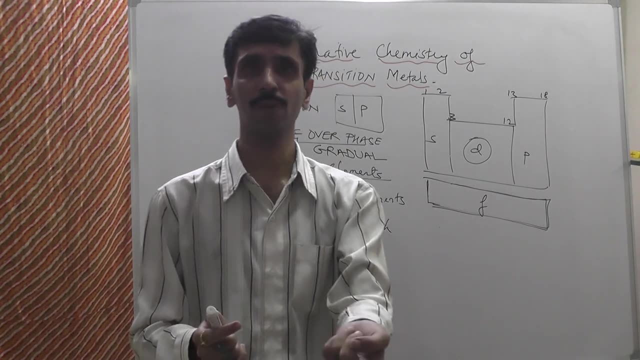 It's a changeover, Okay, a gradual changeover, taking place between the two extremes. Here, the extremes are the metallic to the non-metallic. Okay, that is S block to P block. Alright, So with respect to the positions, I guess you are being very clear that these D block. 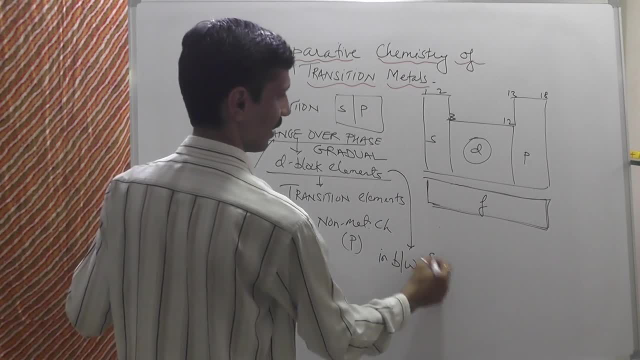 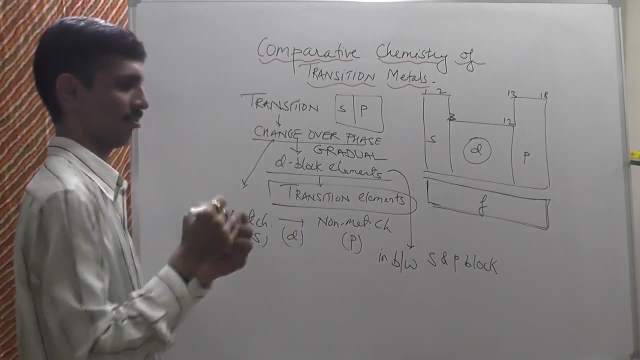 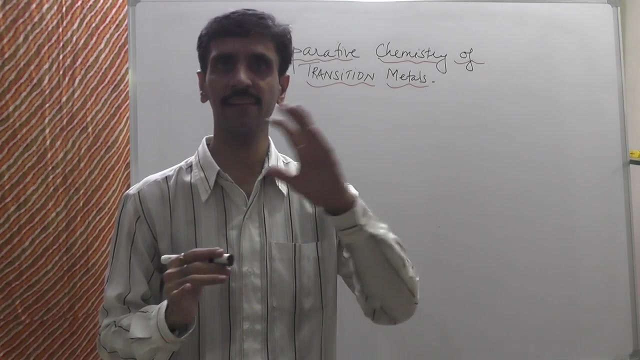 elements are going to be situated in between the S and the P block elements, and hence we use this word, called as transition elements. I hope you have understood up to this very well. I have explained you the transition element concept with respect to the position in the periodic table. 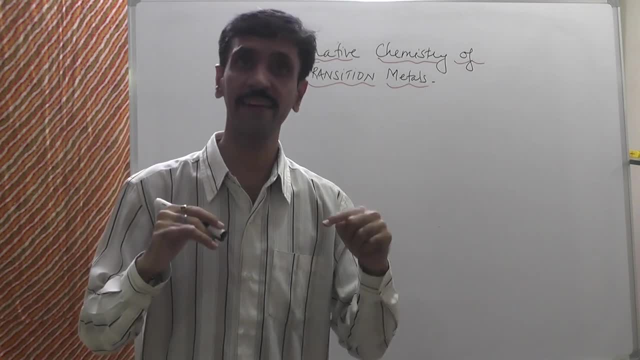 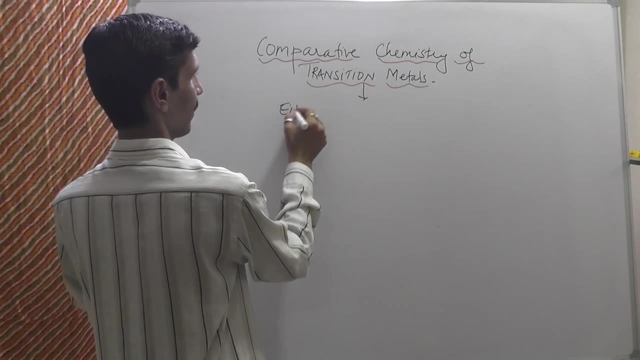 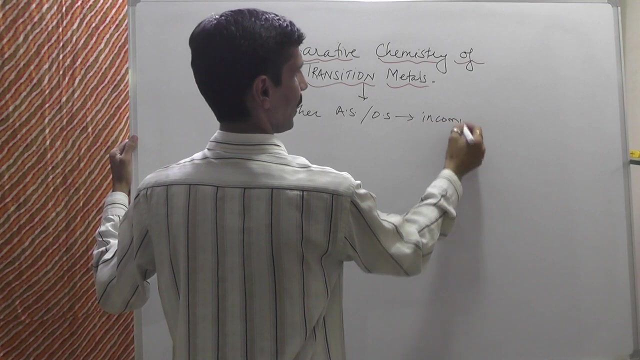 Now we go into the technical aspect of this By taking into consideration the electronic configuration. So what is that? Transition metals are nothing but all those metals which, either in the atomic state or the oxidation state, have incompletely filled D orbitals. 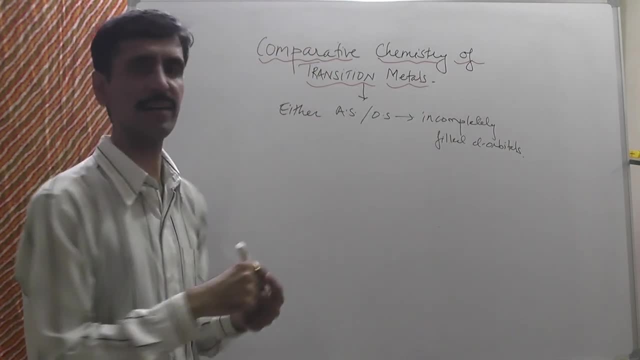 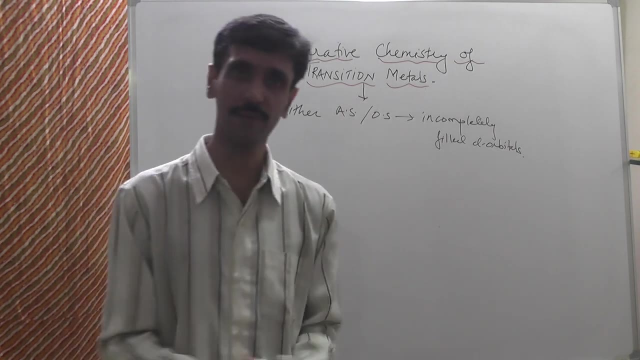 Okay, having completely filled D orbitals, Now I'll try to explain you some terms which are involved in this. Alright, And that marks the end of the introduction of this particular chapter, And that is first thing. is atomic state? Very simple. 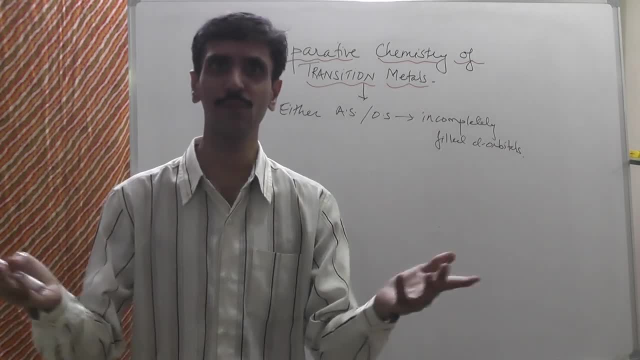 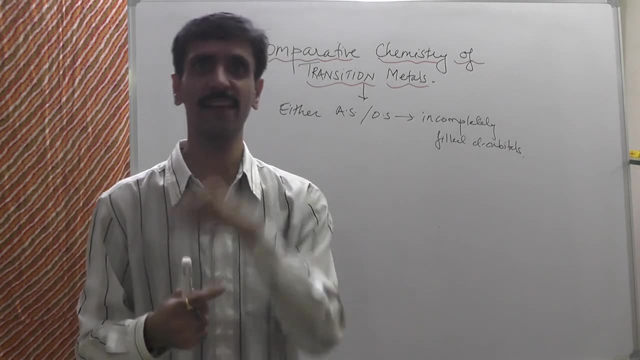 It's a state of an atom And you know very well that atom is what Neutral, So a state where an element is having same number of protons as well as electrons, That is being an atomic state. So whenever I consider an atomic number and write down the electronic configuration on 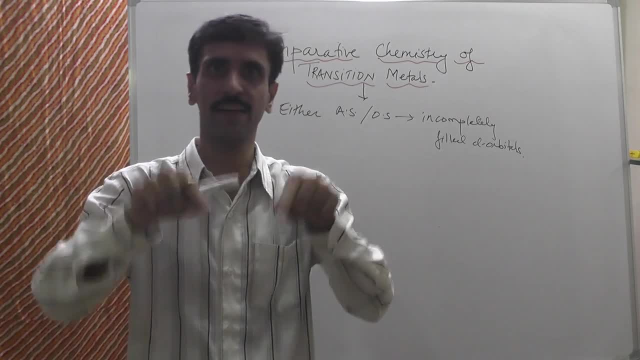 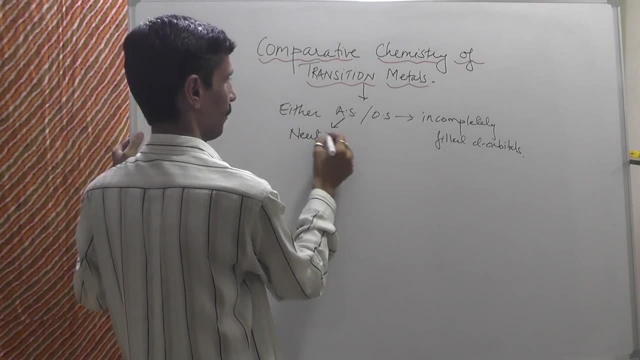 the basis of that atomic number, then I say that that element is in the atomic state, It is in the neutral state. So atomic state means it is neutral Oxidation state. Opposite of that, Opposite of neutral, is what. 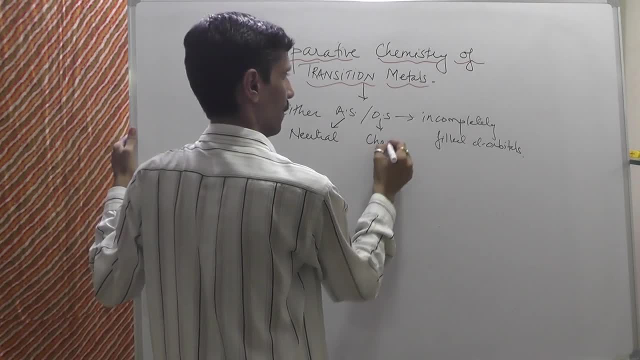 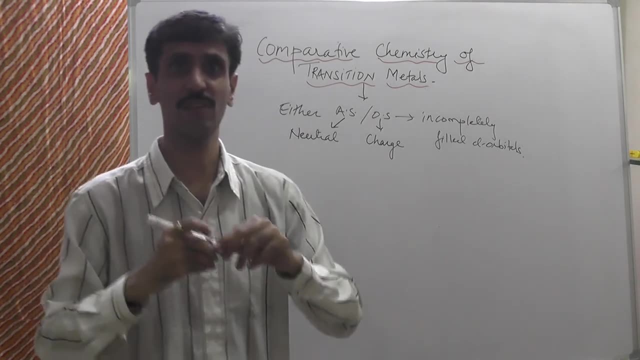 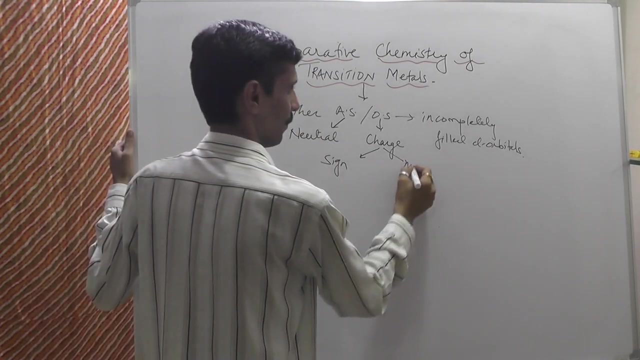 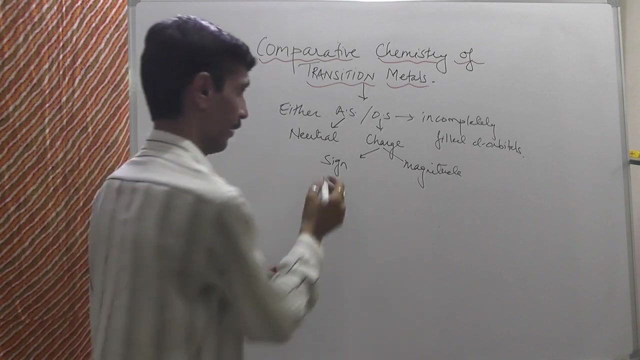 Oh yes, it's charge. Okay, opposite of this is charge. Now, when I talk about charge, it is made up of two parts. The first part is it contains a sign And it contains a magnitude. Okay, Now, when I talk about sign, it can be either positive or it can be negative. 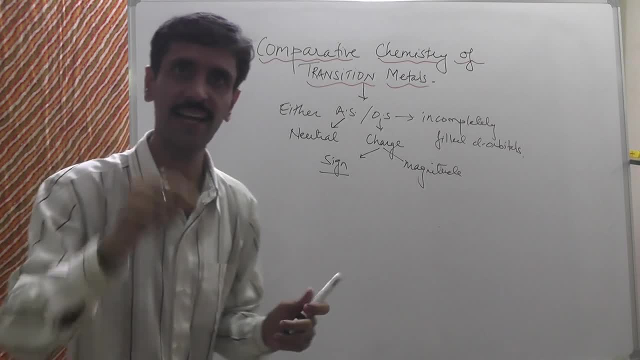 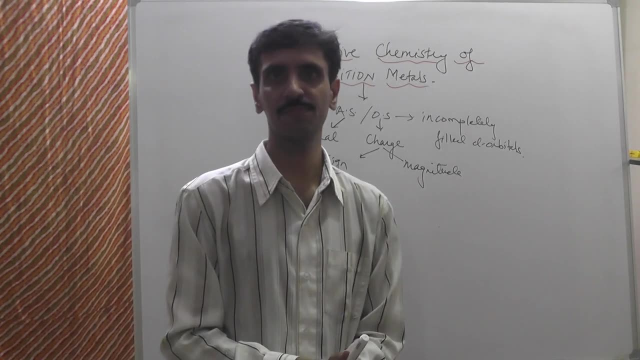 But, as I told you before, that transition elements, all of which are going to show a metallic character, And you know very well, all metals have a tendency to lose electrons Right And when the loss of electrons takes place, electrons are negative. 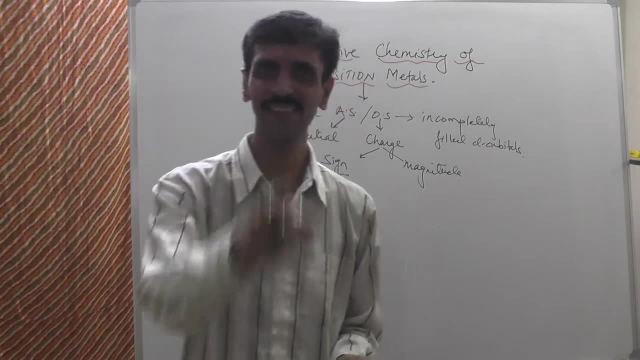 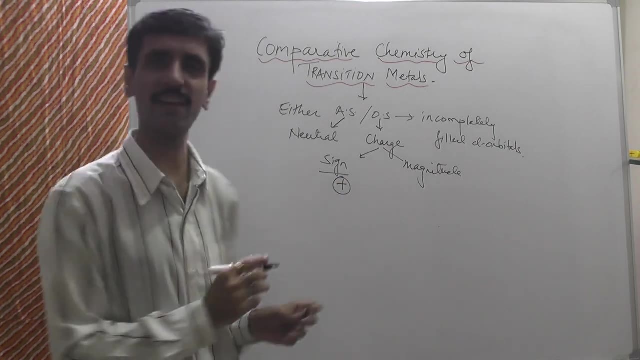 You give away the negativity from your character. See, your character becomes positive. The same thing is over here as well. Okay, So now positive charge is developed, So positive sign always For all the transition elements. Now, magnitude will tell us about the number of electrons lost. 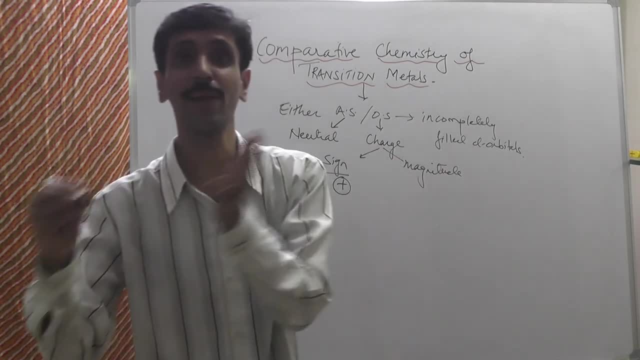 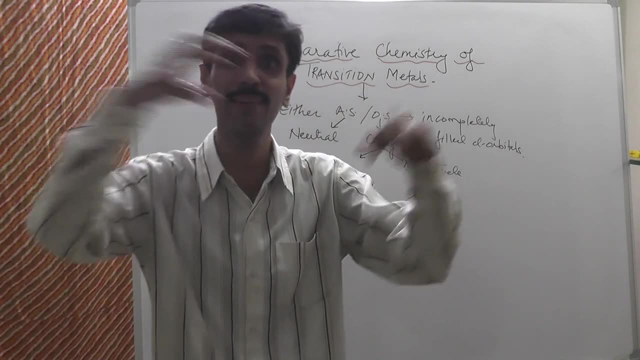 Okay, So that varies, Okay, From element to element. The reason is very simple, because whenever a particular species has a charge, it is only possible when it is going to combine with some other element. So the number of electrons lost, or the number of electrons gained, depends upon the nature. 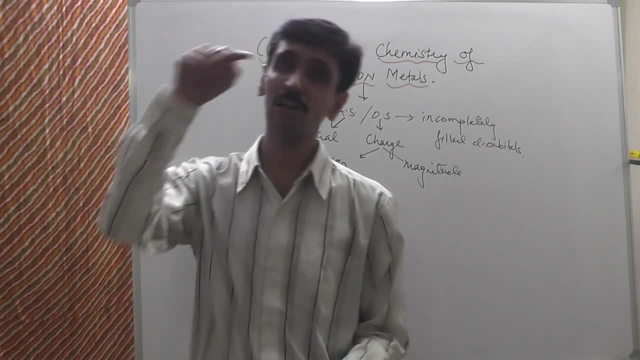 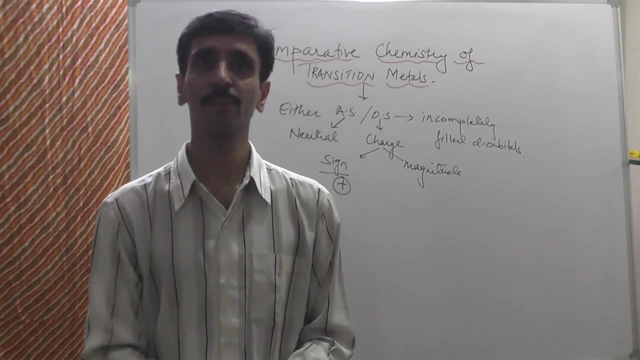 of the element with which it is combining. It also depends upon the reaction conditions. Many times you have seen that the reactants are same but the products are different because the reaction conditions are different. When I talk about reaction condition, I talk about the proportion of the reaction. 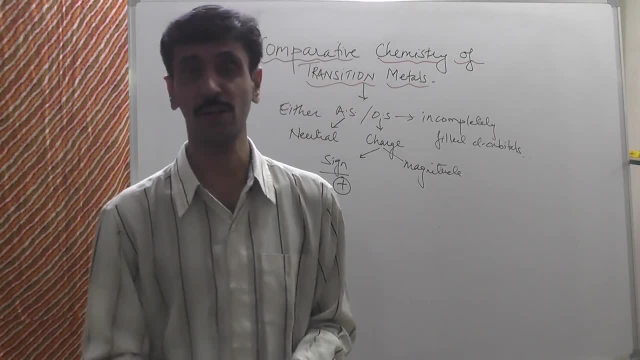 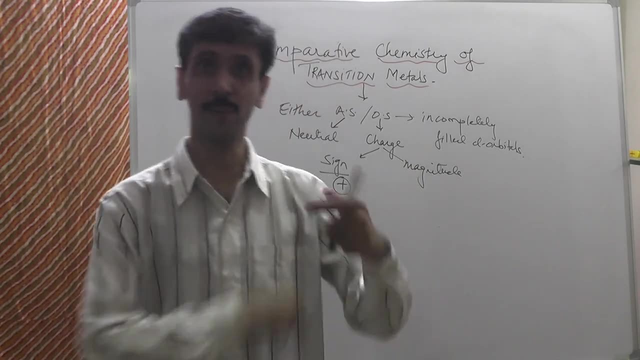 I talk about the temperature, I talk about pressure, I talk about catalyst presence, absence. So all these are the various conditions and depending upon which the products are formed. And if the products are different, the charge also varies of that particular element. 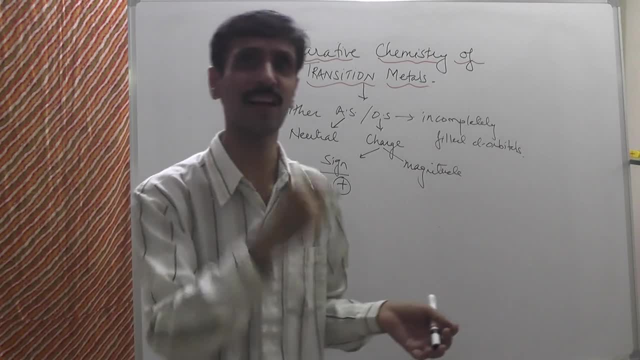 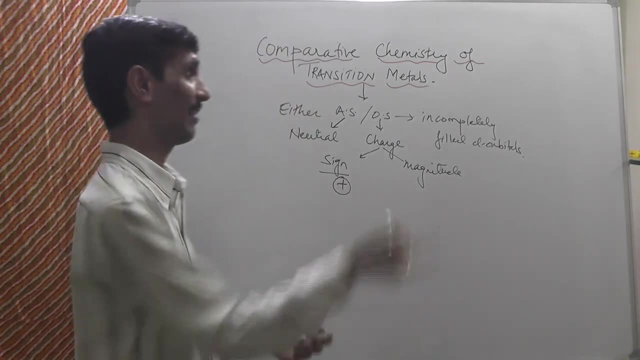 So that is about magnitude, Okay. The number of electrons which are lost, Okay. It all depends upon the reaction conditions and it all depends upon the nature of the element with which these transition metals are combining. Am I clear? But this is always fixed? 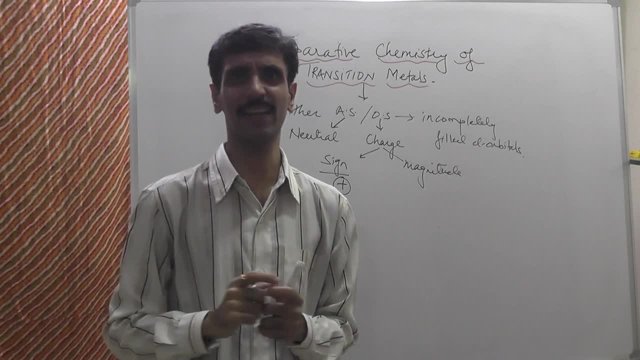 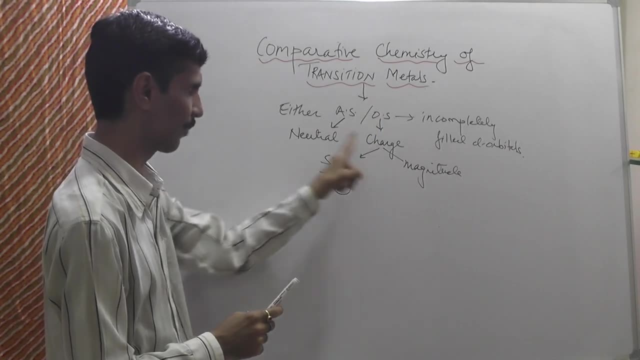 It is always positive. You won't have any transition metal showing a negative charge. Okay, It is not there, So that is what you need to consider over here. So this is about oxidation state charge made up of two parts: sign as well as magnitude. 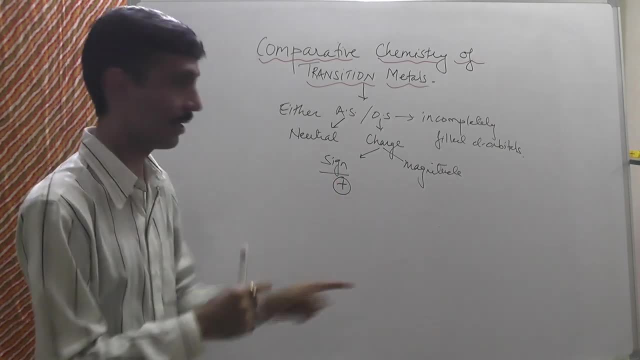 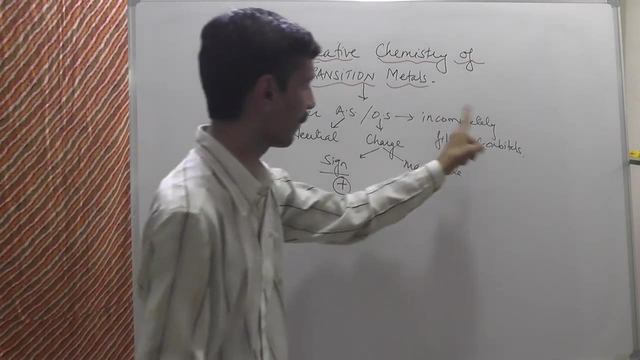 Because they are going to lose electrons. they will always show a positive sign, and magnitude will depend upon the number of electrons lost. Done Fantastic. Now we are going to do this Incompletely filled d-orbitals. What do you mean by this? 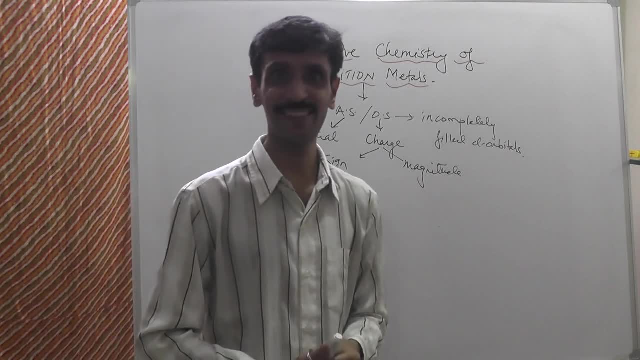 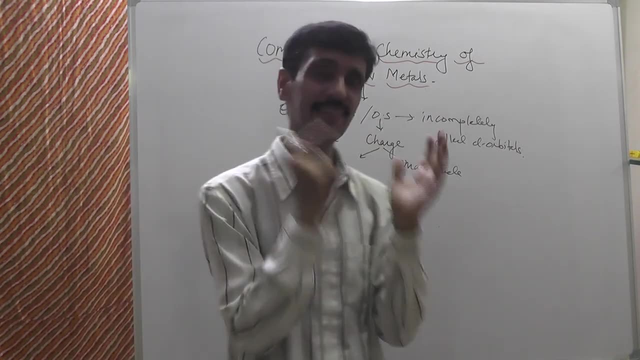 Incompletely filled d-orbitals. Now, what is the maximum capacity of the d-orbital stain? Anything less than the maximum capacity is called as incompletely filled. So now I will consider some cases. Now, first case I consider is d0.. 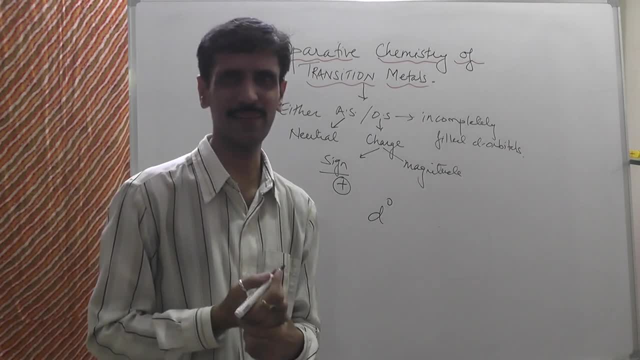 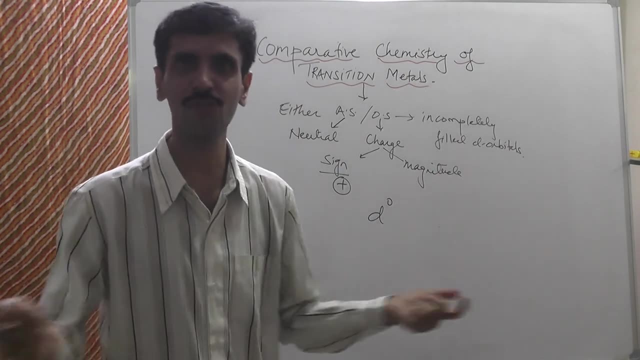 Can I call it as incompletely filled? No, It doesn't sound good, Right, Because no electron is there in the d-orbital In a classroom. also, Suppose if there is not a single student in the classroom, Am I going to say that classroom is incompletely filled? 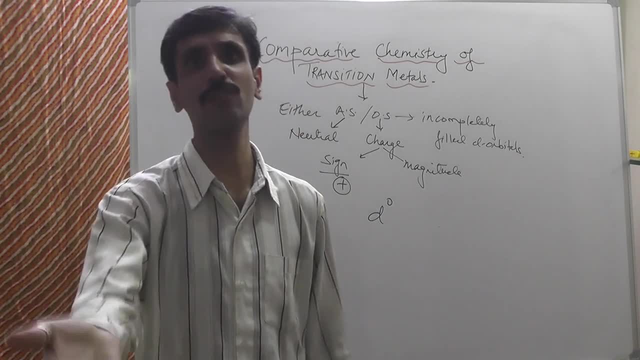 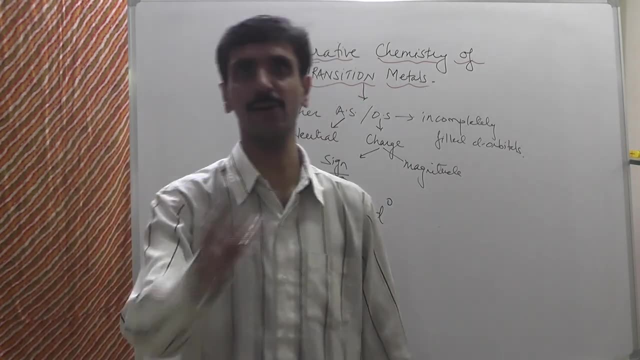 No, Because for incompletely filled there has to be at least one student. Same thing is over here also. For the d-orbital to be called as incompletely filled, there has to be at least one electron in that d-orbital. 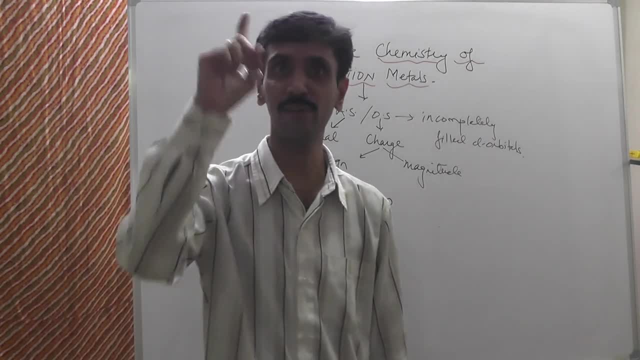 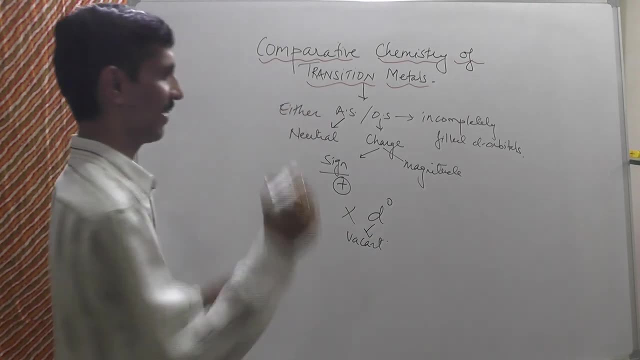 This is 0.. I won't call it as incompletely filled. I will use the word vacant. Okay, So this is called as a vacant orbital. Okay, So I am not going to consider this, because my definition says very clearly. 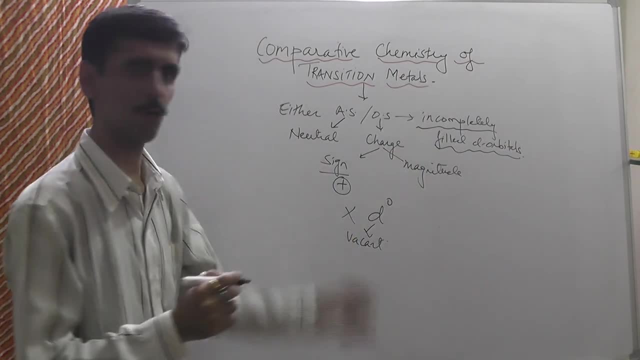 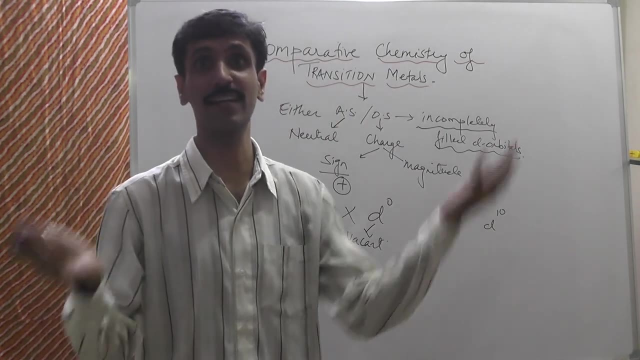 It is incompletely filled a d-orbital, So this is out. Can I call it as detained? No way, Because the maximum capacity of the d-orbital is 10.. Okay, So it is completely filled. It is common sense.